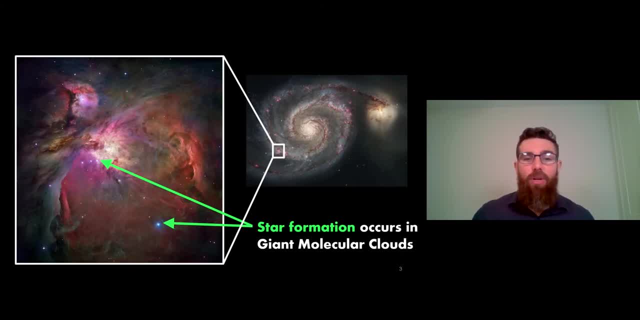 formation process. now on the left hand side i've got a nice image of the orion nebula, which is a stellar nursery where stars have been forming. so i've pointed out a couple of bright blue stars there in the nebula. and on the right hand side you've got a nice spiral galaxy. now star formation. 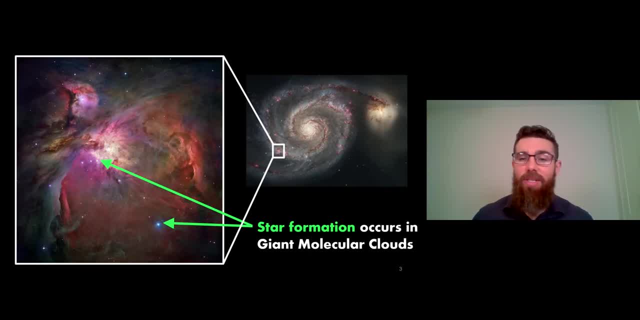 is assumed to occur in these giant molecular classes and those giant molecular clouds are almost exclusively confined to your spiral arms and you can see some of those redder regions in the spiral arms of the actual galaxy and they are corresponding to similar sort of structures to the orion nebula, where these stars 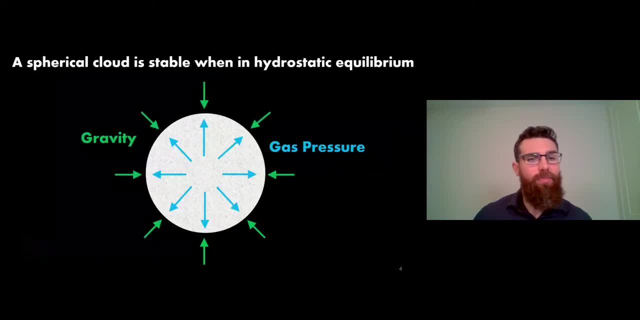 are forming. so we're going to assume that is our starting point and, for simplicity, actually we assume the cloud is spherical, but we know that in the real world it's not. but it makes the mathematics and the assumptions more simple, so we're going to assume that's the starting point. 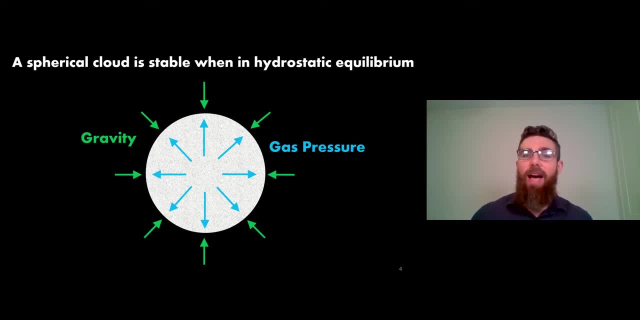 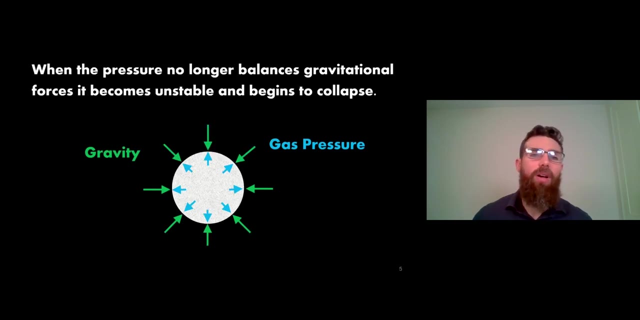 so let's take a spherical cloud, and it is stable when it's in hydrostatic equilibrium. so what that means is that your gravitational forces are being balanced by some outward gas pressure. so it's static, it's not collapsing and it's not expanding. however, at some point, 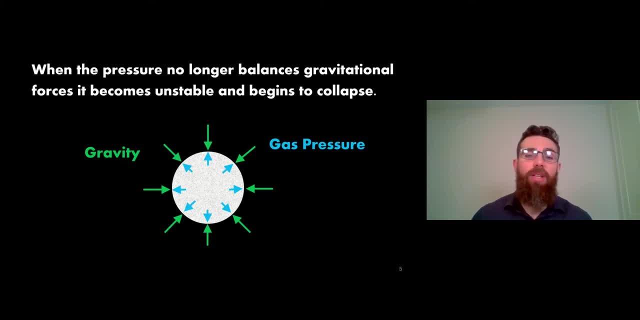 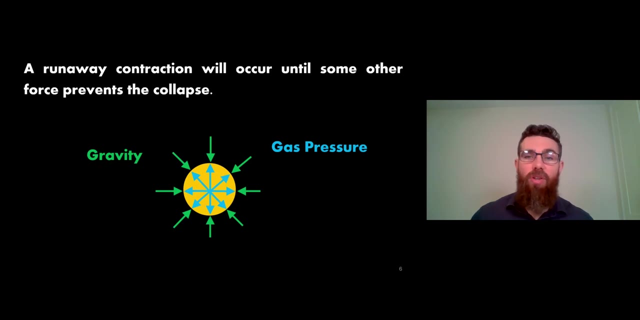 one of those two forces may not equal the other, and in the case of a collapsing cloud it means that the gravitational force overcomes this gas pressure, so you end up with a collapse. it becomes unstable to gravitational collapse and starts to collapse. you then get a runaway contraction and it just keeps collapsing. but there is something that then will limit that. 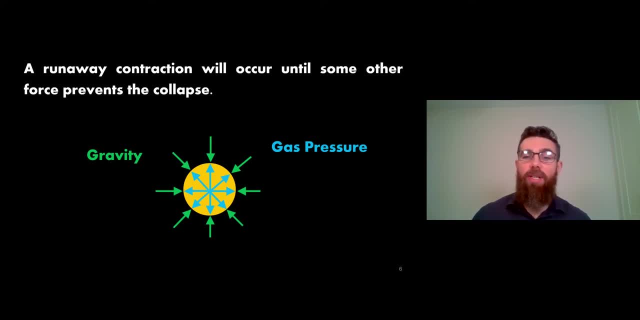 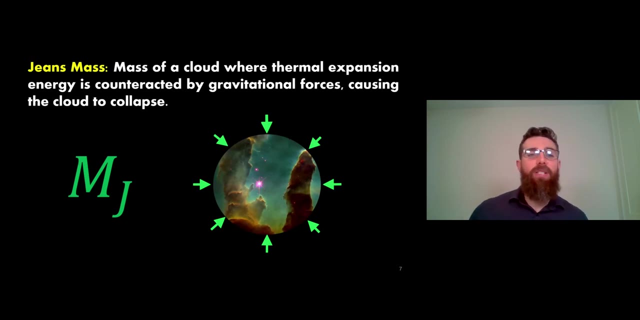 collapse. so at some point those forces are going to start to balance out again. that gas pressure increases and you're somewhat limited and at that point there we're getting close to the formation of a star at the center. now what we can do is we can basically work out an expression for the mass of a cloud, at what point it would become. 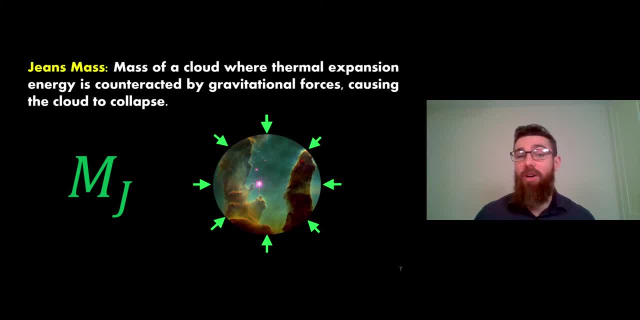 unstable to this gravitational collapse. so it has to be a certain size for it to be unstable to gravitational collapse. so we can work out the jeans mass, which is the mass of the cloud where the thermal expansion energy is counteracted by gravitational forces causing the cloud to collapse. so if you've got a mass larger than this jeans mass, it means that it's going. 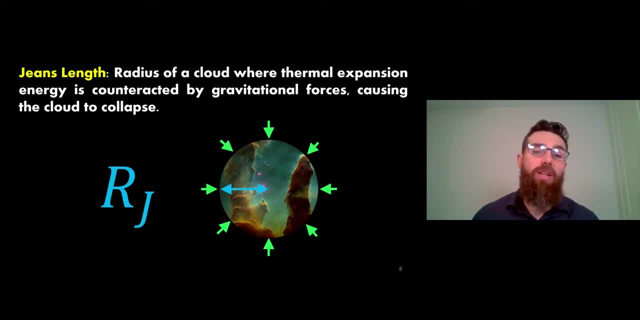 to be unstable to collapse. you can do the same thing for its actual radius. so the jeans length or jeans radius is the radius of the cloud again, where the thermal expansion energy is counteracted by the gravitational forces and therefore you get a collapse of the cloud. so if your jeans 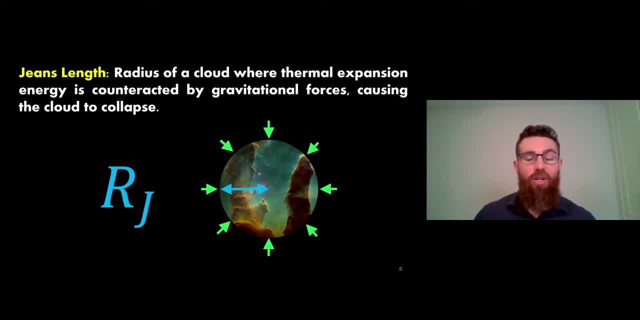 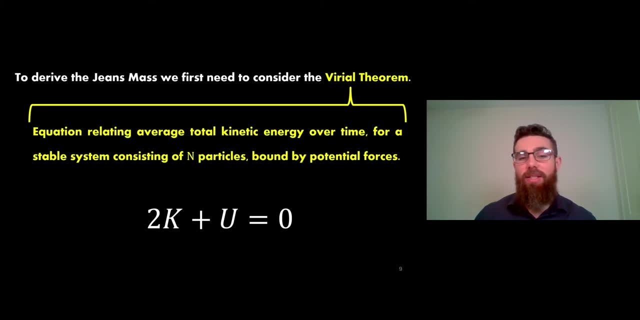 length or radius is larger than this particular value, you're going to get a collapse of the cloud now. to work that out, you can use this particular theorem, and this theorem is just an equation that relates the average total kinetic energy over time for a stable system of n particles, which is bound. 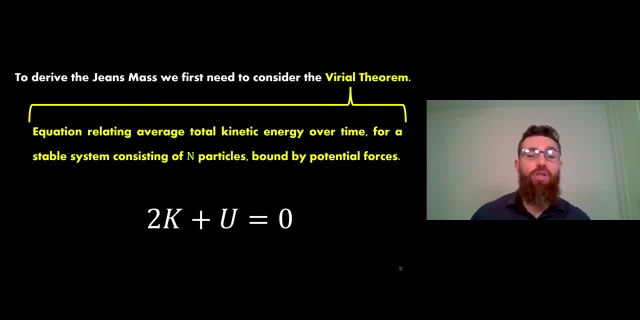 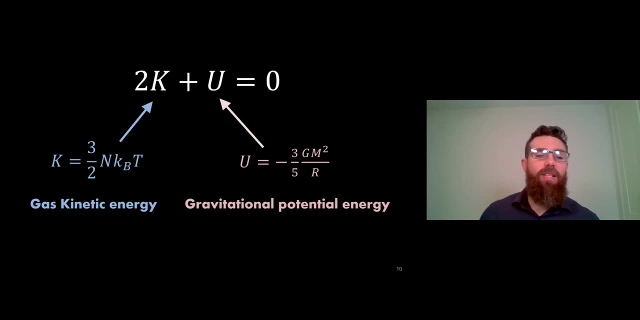 by potential forces, which is your gravitational forces. so here you've got 2k, which is your gas kinetic energy plus the gravitational potential energy, which equals zero. now we can. we know we have some expressions for those so we can put them in. so on the left hand, 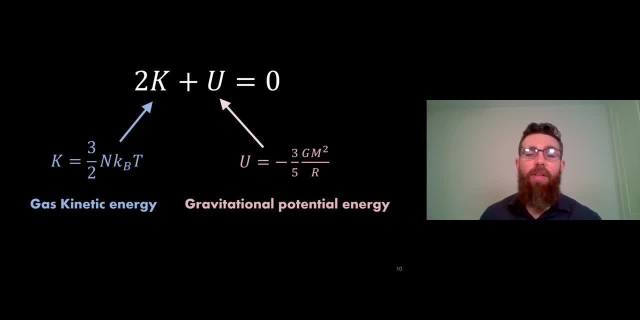 side. there you've got the gas, kinetic energy and then you have the gravitational potential energy. now we want to work out m and r, because that will be our jeans radius and jeans mass. now i'm not going to do the full derivation here. i've got other videos which go through those derivations in the 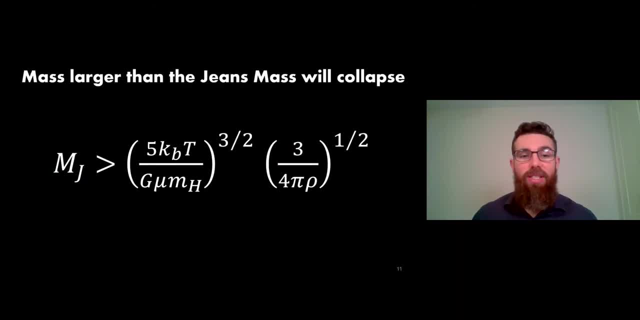 full. but if you do all of that and rearrange it, you should get an expression for the jeans mass that looks a little bit like this now, in that you've only got two variables, so t is your temperature, that's the temperature of the cloud, and then you've got rho, which 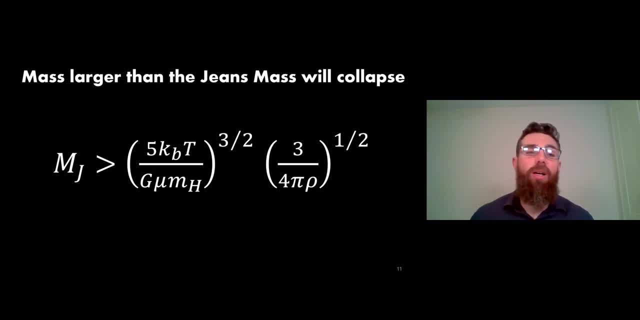 is your density, so they're the only two variables there. and if your jeans mass is larger than this, so your mass is larger than the jeans mass- you're going to get a collapse of the cloud, and what that actually tells you is that cool dense regions are favorable to collapse, because if our jeans mass is proportional to the temperature, to 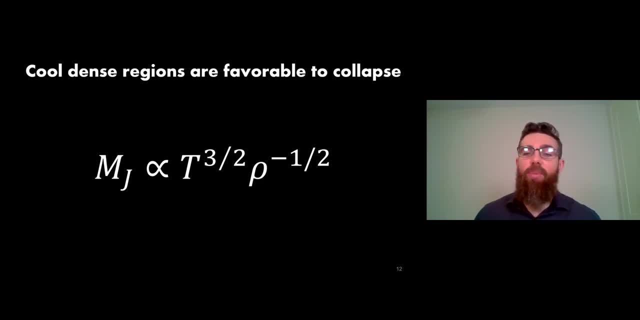 the power of three over two and the density to the power of minus one over two. then as the temperature increases, we to have a larger genes mass, We need a larger cloud for it to be susceptible to collapse. And again with the density, actually as the density increases, our genes mass will decrease. 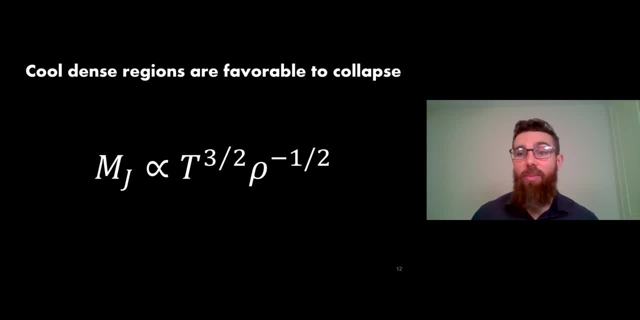 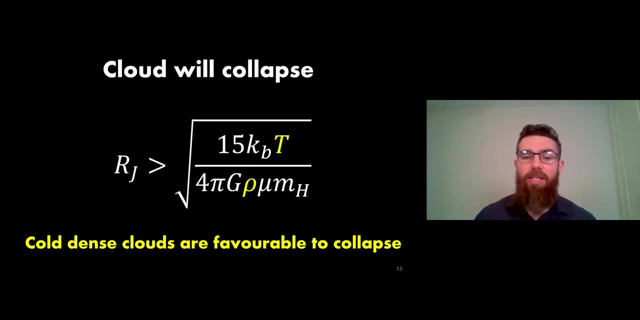 So that tells us that cool, dense regions are going to be favourable to collapse, And the same is true, actually, if you look at the radius as well. So again, you only have that temperature and density, And it just tells us that cold, dense clouds are going to be favourable to collapse. 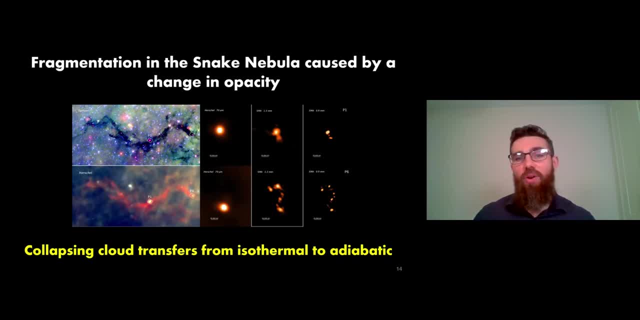 Now we've just assumed that you've got this large spherical cloud that's collapsing to form a star. But again, in the real world, when we look at in space, we don't see that. you're not just going to get a large cloud collapsing into a star. There's some fragmentation that's occurring, So stars 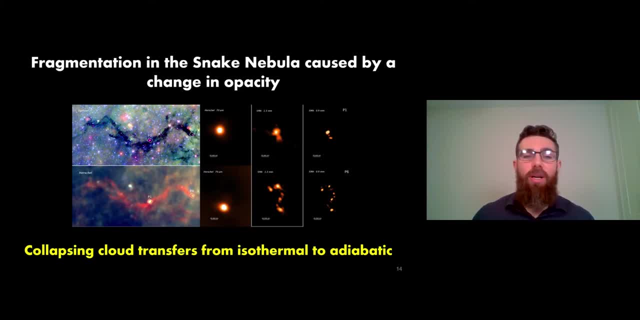 forming in clusters. So something must be causing a process that causes that fragmentation of the cloud as it's collapsing. So here you've got this snake nebula And if you look at that in different wavelengths you can see that it's in a cluster, And if you look at it in different, 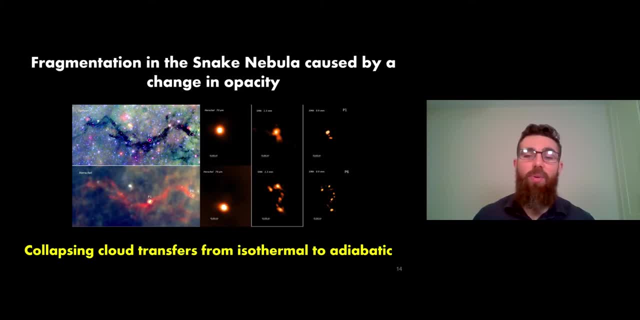 can see that you've got clusters of stars occurring. you can see them zoomed in at different wavelengths on the right. but what's actually happening here is, as that cloud is collapsing, it transitions from an isothermal collapse to an adiabatic collapse. so that means that that gravitational potential. 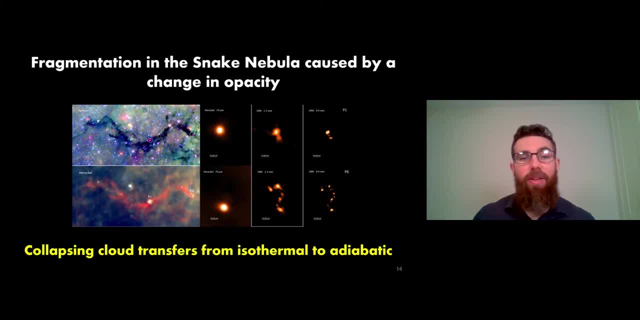 energy begins to be irradiated into the surroundings and then, at some point, the cloud becomes opaque and it's held within the actual clouds that the cloud begins to heat up and at that point it becomes adiabatic, and that is one of the processes that can cause this fragmentation. 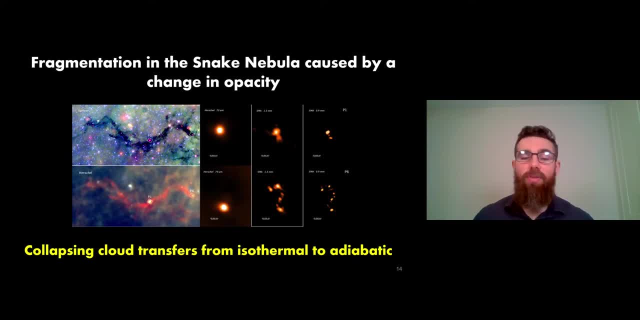 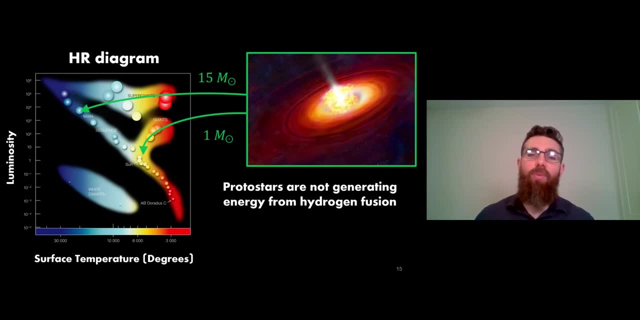 there's other things that's happening there as well, but this is part of it. now, once we've got to this sort of stage, we've got a protostar. now these are not generating energy from hydrogen fusion in their core. most of their energy has come from that gravitational collapse. 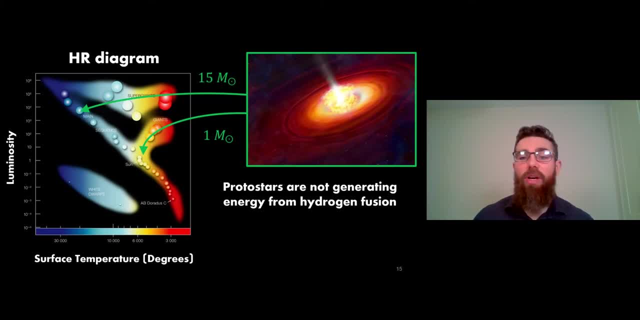 of the of the cloud initially. so they're not quite hot enough to undergo that hydrogen fusion. they're not. they're not fully collapsed, so they are kind of they're not in a fully hydrostatic equilibrium state at the moment. there's still some contraction there of the cloud and the protostar. but the interesting 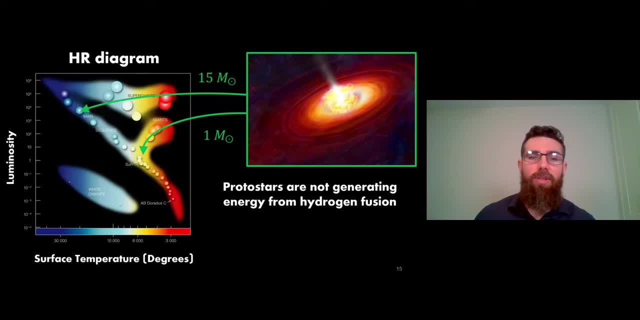 thing here is they're not on the hr diagram at the moment, but they kind of move left onto it. they come onto it from the right hand side. now, depending on the mass of that protostar, it takes a slightly different route. so the smaller protostars when they drop down onto the main sequence. 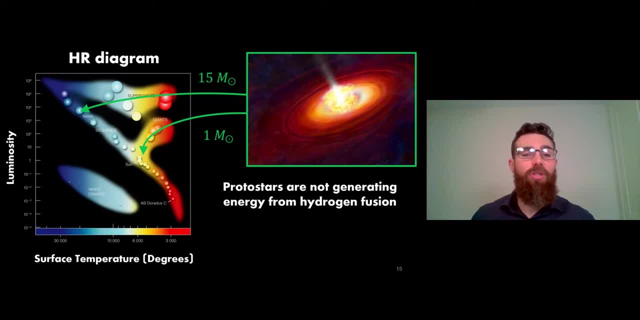 they will actually take a more vertical route, whereas the larger ones it's more horizontal and that's to do with more their size and their luminosity. so they're the bigger protostars are already quite close to the upper limit of luminosity, which we'll mention in a little bit. 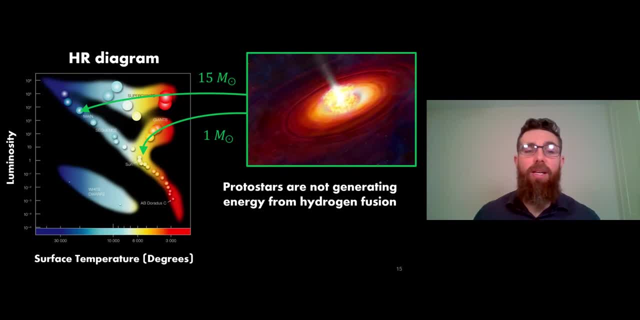 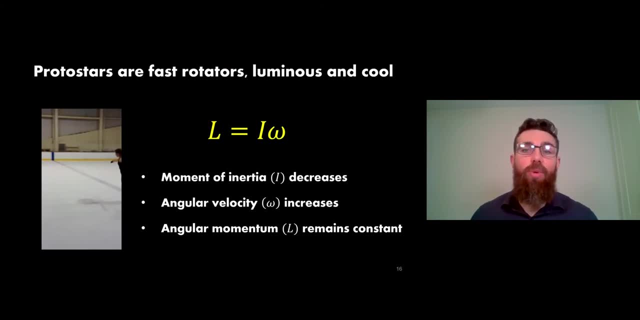 so the size denotes their absolute route. they take on the hr diagram and onto the main sequence. now, protostars are quite fast rotators. they're luminous and they're cool. they're luminous because they're actually quite large, because they haven't fully collapsed yet, and they're not quite large because they haven't fully collapsed yet. 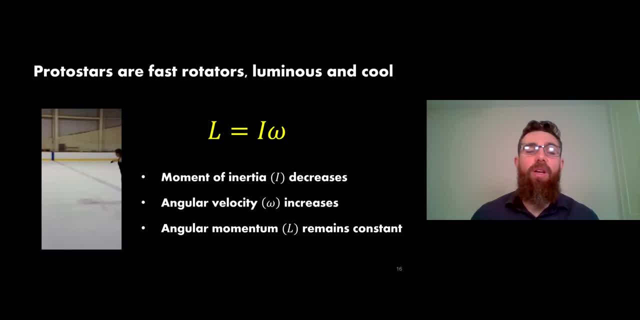 and they have fairly cool surface temperatures. but because they're fast rotators, we've got this cloud of gas that had some kind of net rotation to start with and as it's collapsed, to conserve that angular momentum, they actually have to rotate faster. so by collapsing that moment, 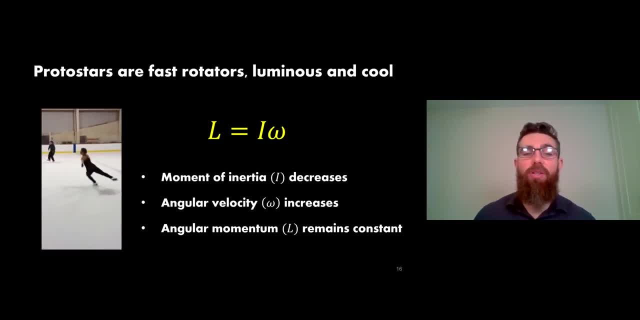 of inertia has decreased, you've moved that mass towards the center of the rotation axis. so therefore, to keep your angular momentum the same, your angular velocity has to increase. so this is why our younger stars are typically going to be quite fast rotators, and you can see a video there giving a visual example of that. someone who's ice skating and has their 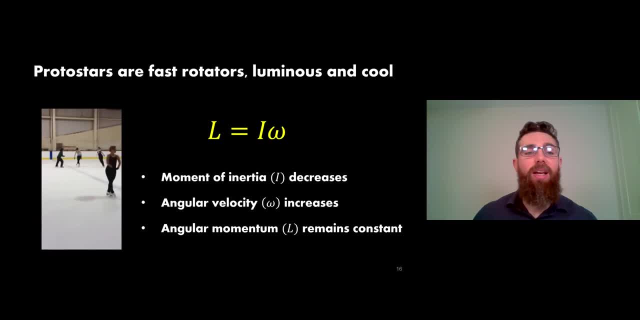 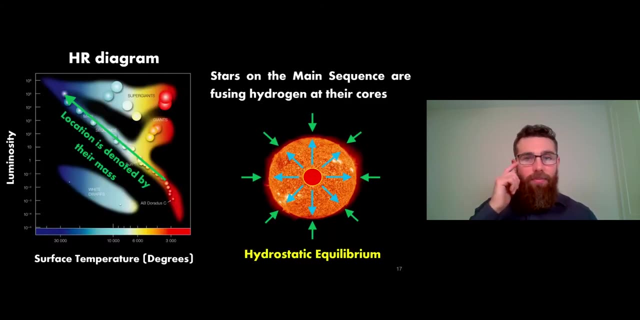 arms out and they pull them in close. they can increase their rotational speed purely by doing that, because the angular momentum hasn't changed, but because they've decreased their moment of inertia, their angular velocity does increase. that's the same with stars. now stars on the main sequence are fusing hydrogen at their core, so they've got a central core which 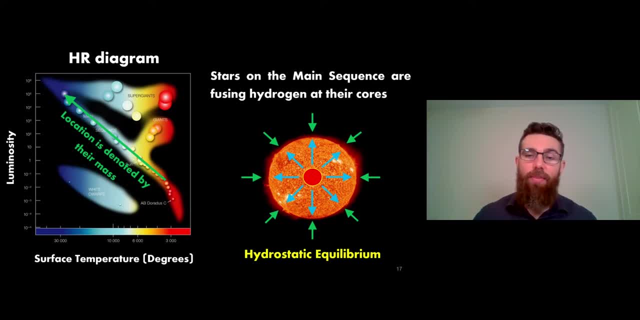 is now at the right temperature to fuse hydrogen into helium. they're in hydrostatic equilibrium and they're quite happy sitting there for a fair chunk of their life. really, now, depending on their mass, it depends where they are in this main sequence. so on the hr diagram. 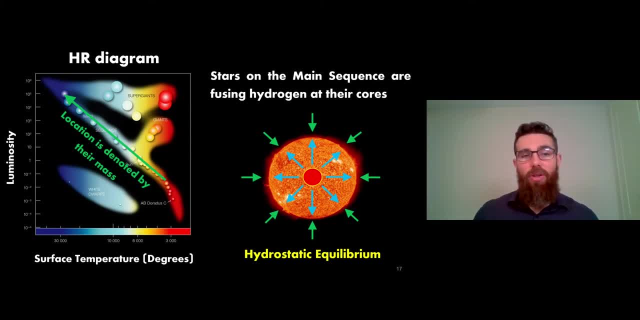 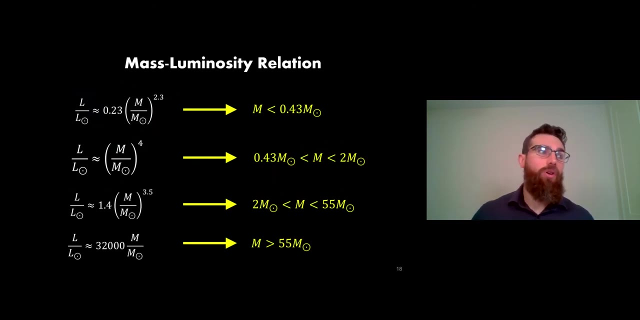 you've got this diagonal right down the middle and the larger the star, the higher up that they sit at that main sequence and the Sun is kind of about a third away from the bottom. really now there is a mass luminosity relationship, so the bigger the star, the more luminous it. 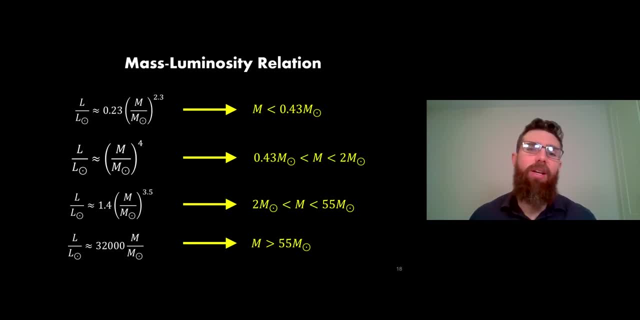 the sun has turned into planet these days, but it's not as straightforward as just having a single relation there. so what you actually have is is: for the smaller stars- you've got this top expression here, so you've basically got mass is to the power of 2.3, and then for Solar mass stars, it's about to the power of 2. point 3. 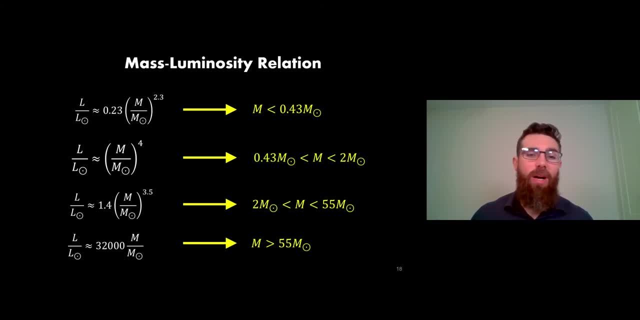 Because they appear to be predictions. more like increasing Earth's Fastene, they show that they're getting higher and higher, and then for solar mass stars it's about to the power of four, And then it changes again for stars greater than two solar masses up to 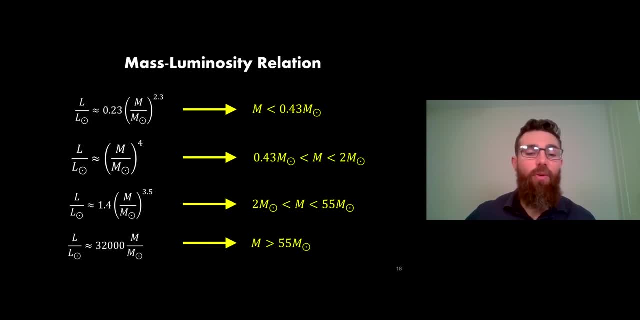 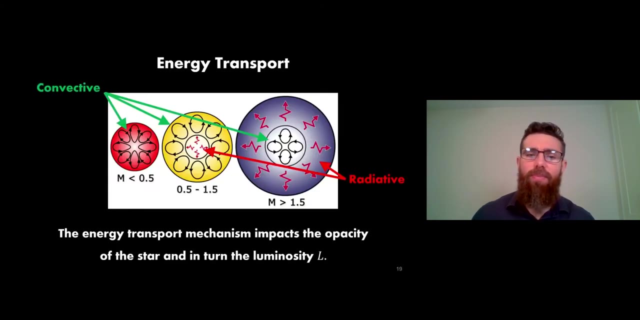 quite large stars And, at the very bottom, your most massive stars have a different mass luminosity relation as well. Now, what's actually causing or driving that particular relation? Well, it's predominantly down to the energy transport mechanism. So if it's convective or radiative, 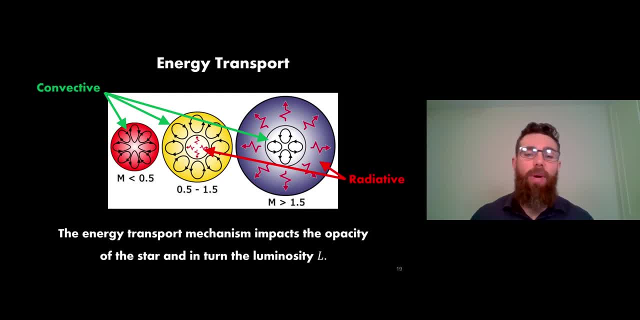 then it's going to impact their luminosity. So the energy transport mechanism impacts the opacity, how opaque the star is, And that in turn alters your luminosity, Because if your star is quite transparent or quite opaque, it alters how luminous it is. So the actual energy coming from 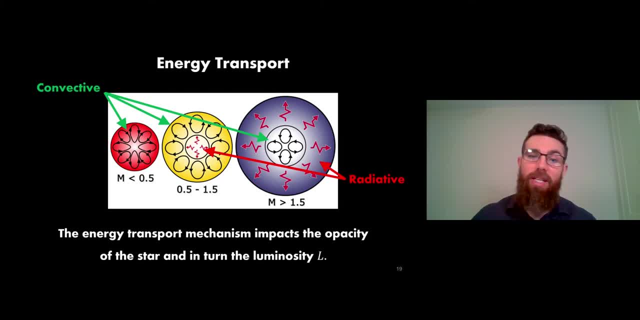 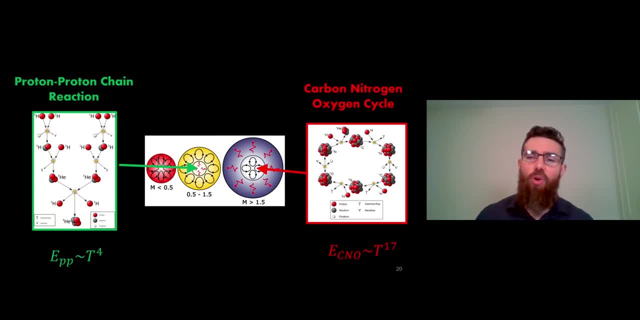 the surface, And it's down to the way that energy is transported internally. Now, why does that actually occur? Well, just to point out a couple of things that's occurring in the central core which might give you an idea as to why you might. 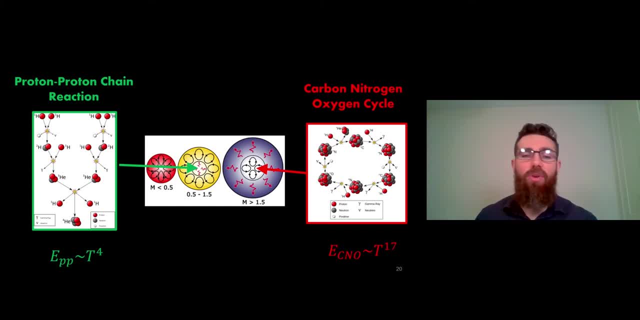 have a convective core or a radiative core. So for solar mass stars like our sun in their central core, the most dominant energy mechanism is from the proton-proton chain reaction. Now the energy production rate from that particular reaction scales with temperature. 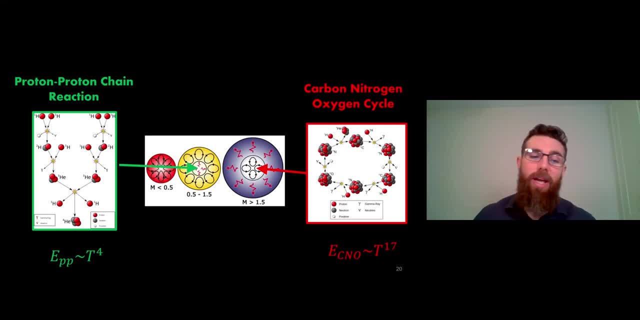 to the fourth power. So if you increase the temperature, then the energy production goes up by that amount. Now, in the larger stars they're higher. So if you increase the temperature, then the energy production goes up by that amount. Now in the larger stars they're higher. So if you increase the temperature, 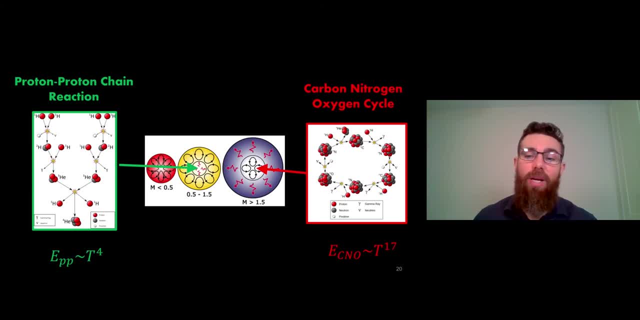 you increase the energy production by a lot more, So actually it's to the 17th power, this energy production rate as you increase the temperature. Now, what that does is it causes a very large temperature gradient, which then initiates the convection because of that. 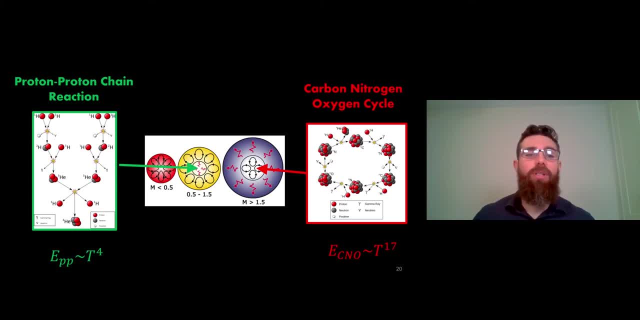 temperature gradient. So actually it causes a very large temperature gradient, which then in the It depends on the dominant energy production that's actually occurring in the star. as to whether you get that or not, That then impacts how opaque the star is and also the luminosity as well. 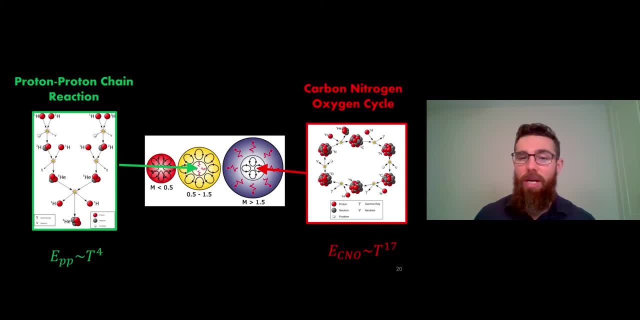 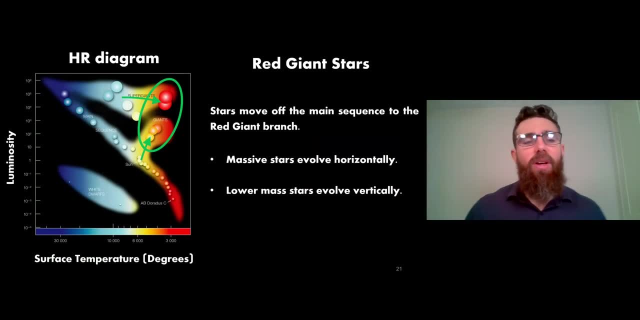 So that's only a brief overview, but it gives you an idea of what's happening in the core and why it changes for different stars. Now, with red giant stars, once they've finished the main sequence, they finish that hard infusion in their core. 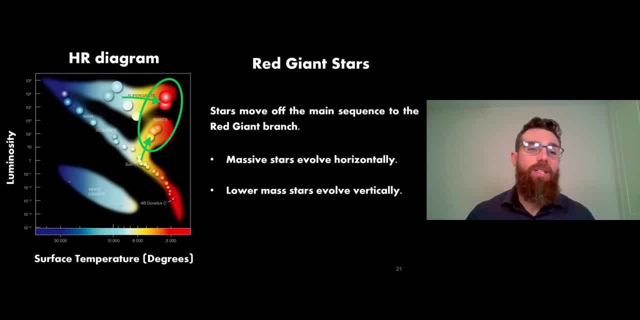 Most stars will go into a red giant phase. So they move off the main sequence to the right or to the upper right, But depending on the size of the star they take a slightly different route. So solar mass stars, they almost go vertical up into this red giant phase. 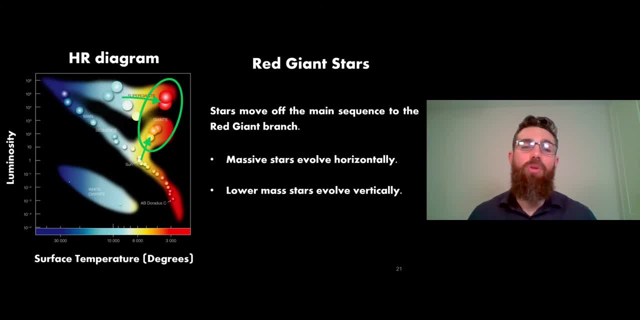 But the larger, more massive stars take a more horizontal route, So they just move to the right from where they were off the main sequence. Some of the very, very large stars actually don't have a red giant phase because they don't actually cool down enough to appear red. 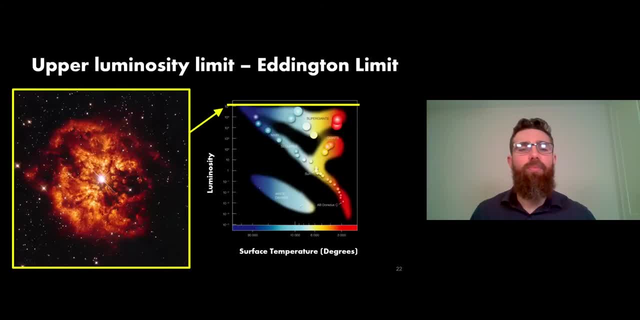 So they actually never get that red giant phase. Now the reason why the larger stars don't get any more luminous- because they can get a cooler surface temperature but they don't get any more luminous- is that they're already pretty close to the Eddington limit. 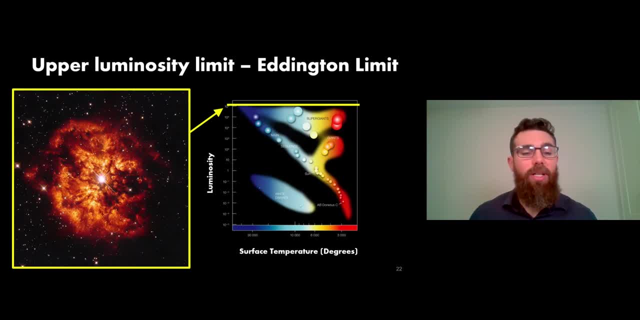 So again, I've got another video that explains that in a little bit more detail. But on the left hand side you've got a star that is pretty close to the Eddington limit. Now when stars get to that limit they've almost got enough outward pressure to blow. 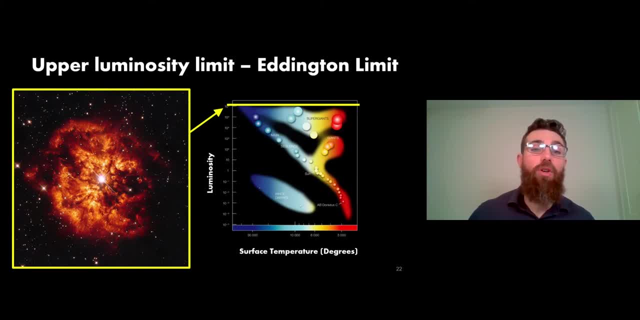 They're out of layers off. So if the stars are too luminous they can overcome their own gravitational forces, So that hydrostatic equilibrium becomes unbalanced again. So there's kind of a hard limit there for the luminosity of a star. 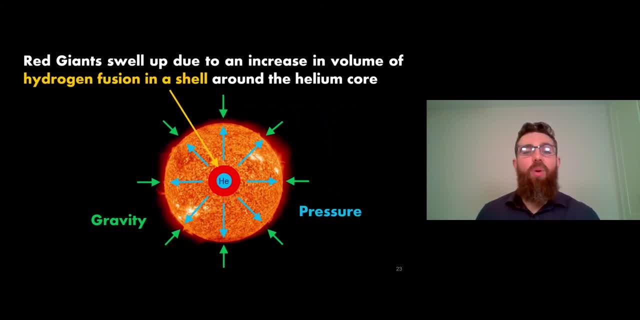 So why did it actually swell up at this point? Well, in the centre they've no longer got a hydrogen core, They've got a helium core which, once the fusion stops that, collapses because there's no counteracting force for the gravity. 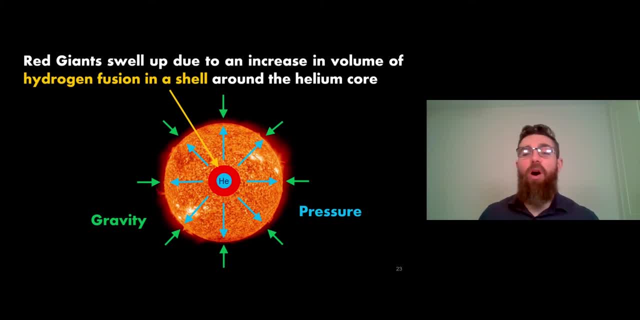 The helium core then heats up again. It allows some hydrogen back in and around the shell, So you've got some additional heat there. You've then got hydrogen in a shell around it which is now at the right temperature to undergo fusion. So what happens is you have this hydrogen fusion fusing shell around the helium core. 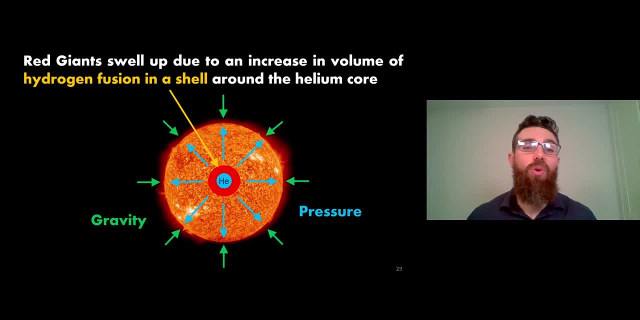 That helium core, so that hydrogen core actually has a larger volume than it originally did in the core beforehand. So it generates a larger volume. So it generates a larger volume And that gives it a larger outward pressure. That then lifts the outer layers further out, because it overcomes the gravitational force, which hasn't changed. 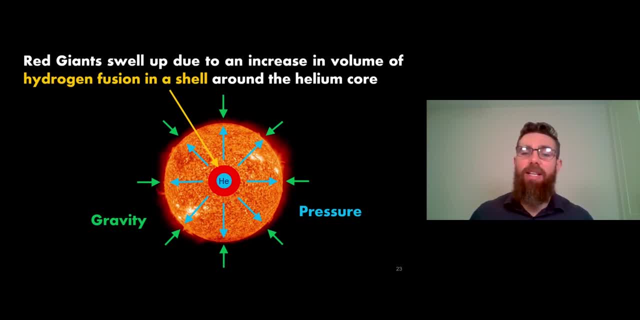 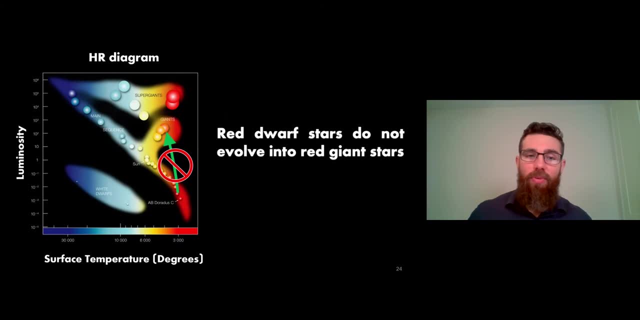 So the star actually swells up because you've essentially changed the outward pressure instead. Now red dwarf stars are at the bottom of the main sequence on the H-R diagram And these do not evolve into red giant stars. So these small stars never go into red giant phase. 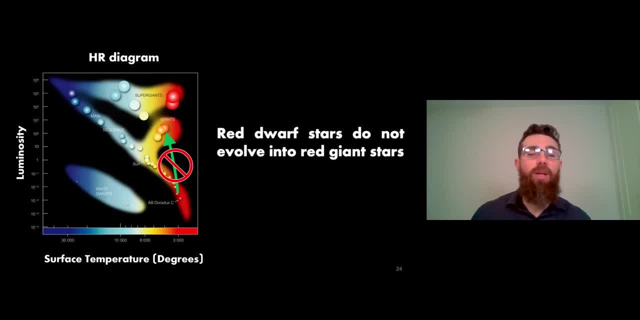 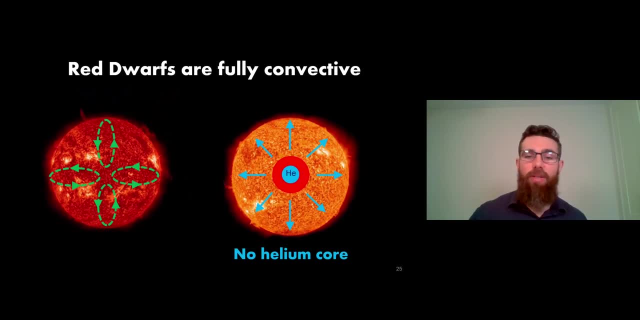 phase. they will always stay as a red dwarf star. Now why is that? Well, actually they're fully convective. so if you look at the energy transport mechanism in a red dwarf star, the whole star is convective. so that means they never end up with a helium core. so they never have that stage where 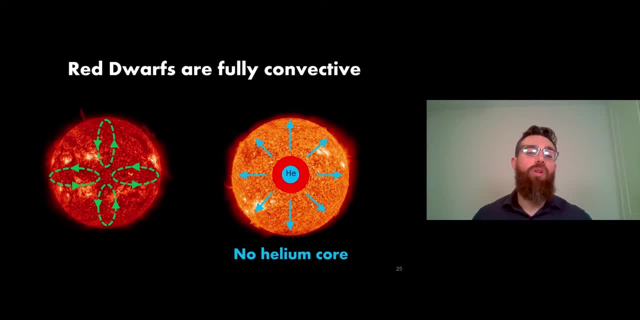 they have a hydrogen shell around the helium core that then undergoes the red giant phase and because they're fully convective, it means that they actually survive on the main sequence the longest. so these will last a lot longer than other stars and they will never have that red giant phase. 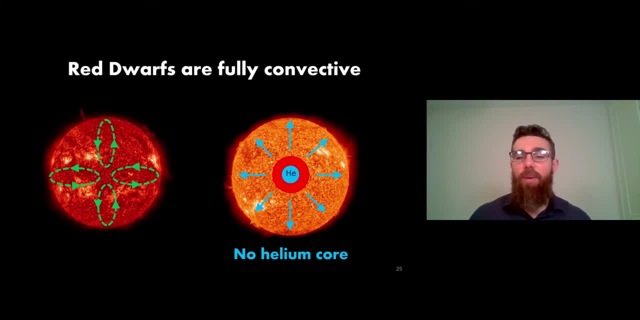 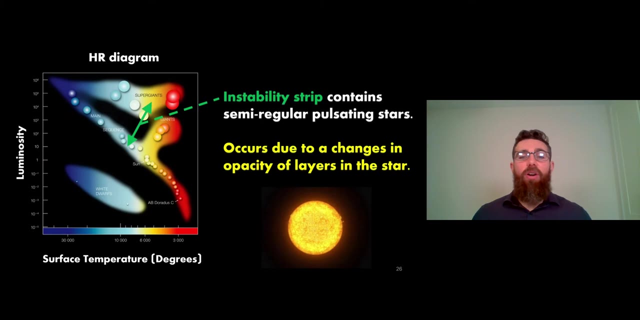 they'll slowly just cool down, and that's what they'd be doing. but it also means they're very efficient, because they turn more of their hydrogen into helium, because they're fully convective and they're circulating it all around in the star. Now, when they're on this red giant, phase once. 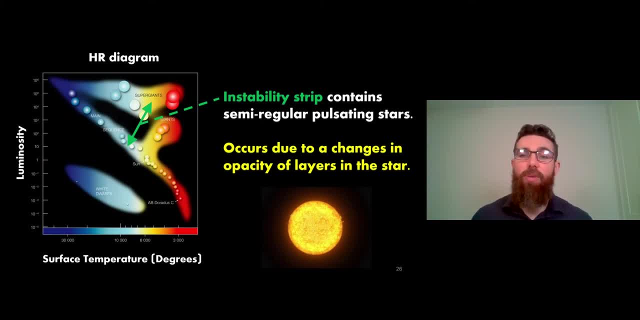 they've moved off the main sequence. they go into this instability strip as well. so this is where you get these semi-regular pulsating stars. So stars here are physically pulsating and it can be regular, semi-regular, but the star will swell up, shrink back down. its surface temperature changes as well. so you can see by looking at the actual 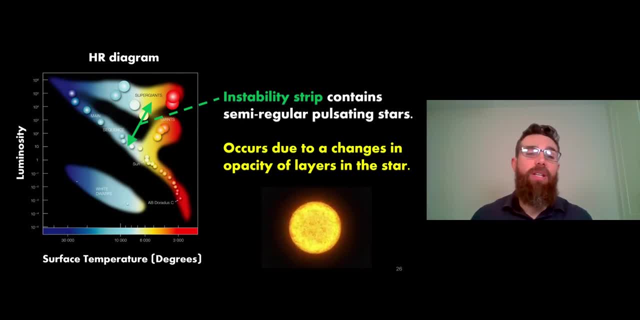 HR diagram that they. it's almost like a diagonal opposite to the main sequence. So as they swell up, they become more luminous, their surface temperature cools and then they do it all over again. This happens because of a change in the on how opaque the layers of the stars are. 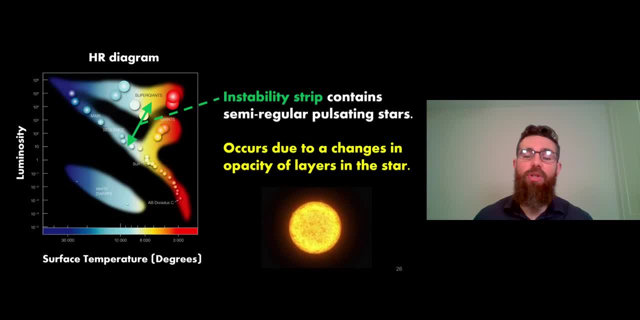 there's actually a few mechanisms occurring here, but predominantly it's due to how that energy is transported through the star. so it swells up, cools back down and you get this nice cycle. and because they're regular, they can be quite useful for finding distances as well. so there's a 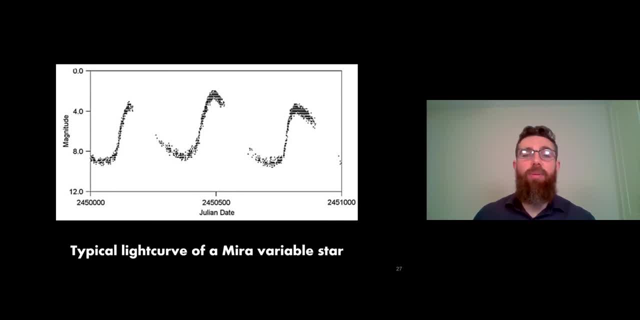 period to luminosity relationship which you can use. if you measure the period that the star is pulsating, you can work out how far away it is by measuring its magnitude or luminosity, and this is a typical light curve of one of these variable stars. Now, the light curve is just the magnitude. 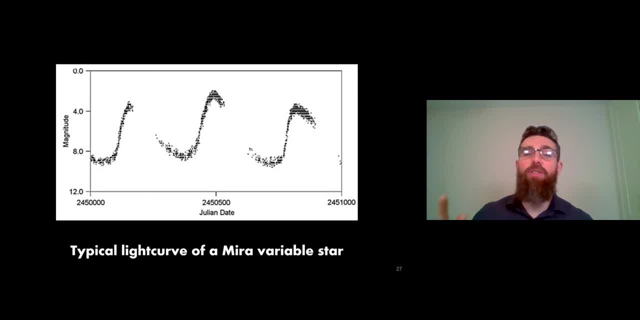 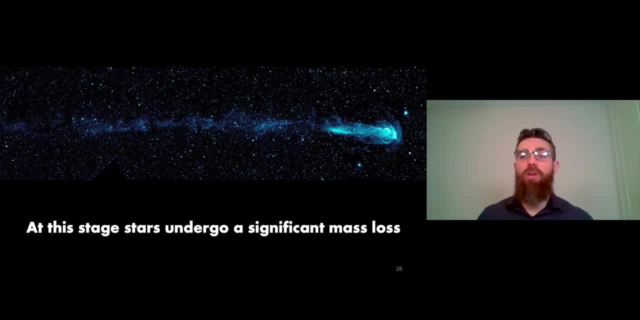 or luminosity of a star against time and you can see you've almost got a nice regular period there. you can easily pick out. Now, whilst these stars are undergoing this particular process, they're undergoing this particular process. they do undergo a significant amount of mass loss, so, as they 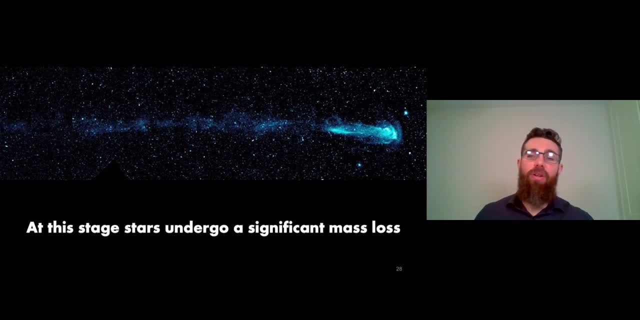 pulsate like this, they can lose their outer layers and you've got a nice image of a star that it's obviously moving through space but as it's doing so, it's losing some of its outer layers and you can visually see the mass loss of these stars. so as they go through the red giant phase and 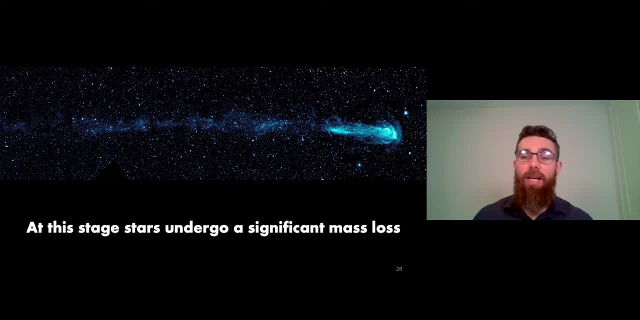 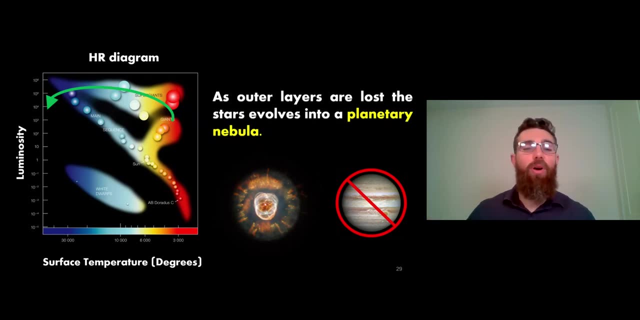 go into the next stage of their evolution. they do lose a lot of mass. Now the next bit is they go into the red giant phase on the upper right of the HR diagram, to a planetary nebula which is across the top of the HR diagram. So here those outer layers are lost and then they're illuminated by 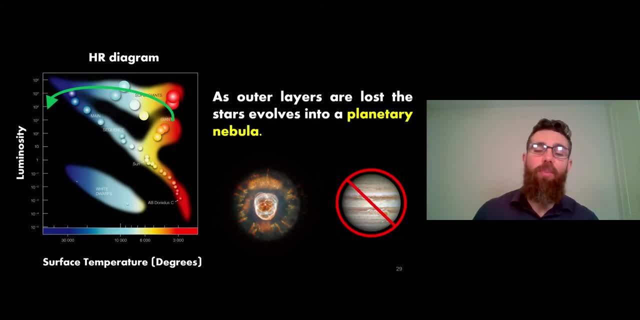 the now hot exposed core. so you've got a nice planetary nebula there. and it's worth noting that these are not anything or nothing to do with planets. it's just purely down to historical observations and what they were thought to look like like when they were first observed. So they have nothing to do with planets, they're just called. 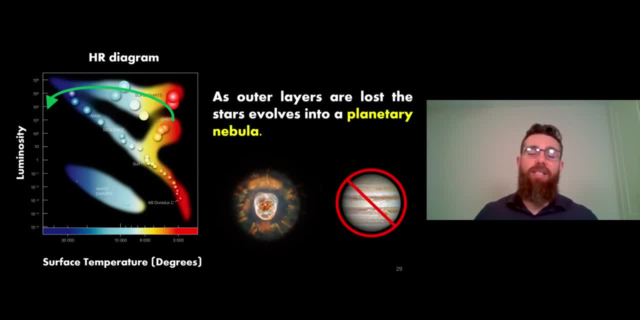 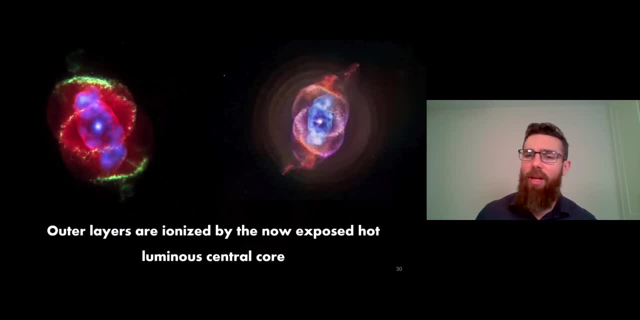 planetary nebulas. But these outer layers are lost and they do create very beautiful looking structures, So you've got a couple more there. So these outer layers are then lost and then they're ionised by the exposed central core. So you've got a very hot central core of 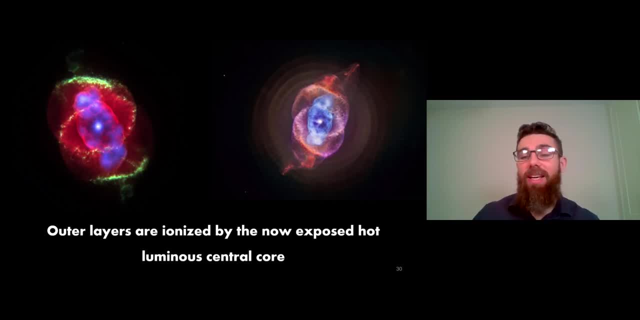 the star which is now beginning to be exposed, That then illuminates or ionises the outer layers, which is what gives you these beautiful looking structures, and which then emit at their own wavelength. So they become quite luminous at this point And they obviously their surface. 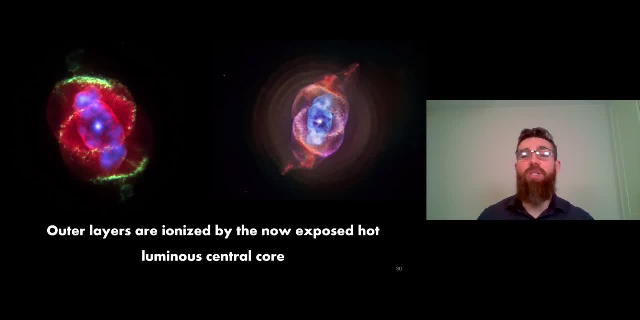 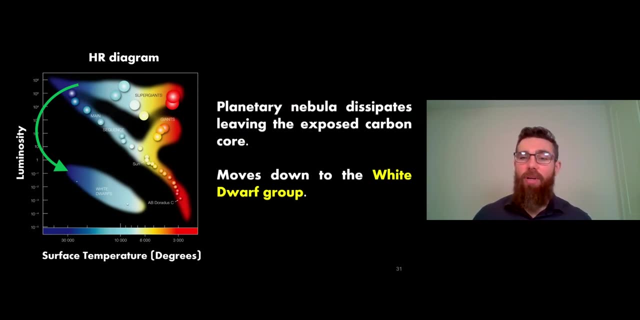 temperatures increase because we can now see their central cores, which is why they take that route across the HR diagram. Now, once they've done that, the planetary nebula dissipates. it then leaves this exposed carbon core, carbon oxygen core, and it will move down into the white. dwarf group. So they've become less luminous, but they've become quite luminous. So they've become quite luminous, but they've become quite luminous, but they've become quite luminous. So they've become quite luminous, but they've 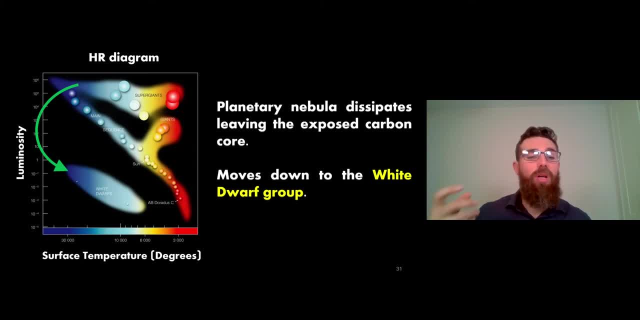 become quite luminous because those outer layers have been lost. You've only got that very small central core left. So yes, they have very high surface temperatures, but because they're very small, their luminosity is not that great. So that's why they come down on the HR diagram. 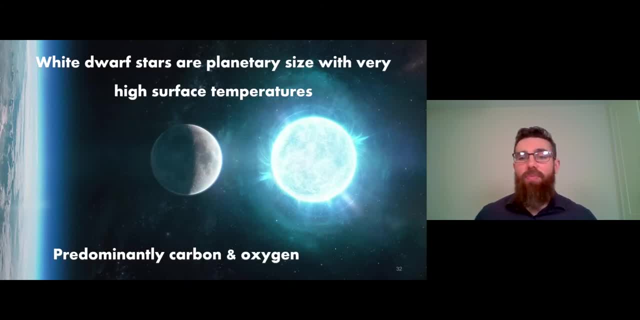 Now, the white dwarf stars are typically planetary size, So this is an illustration of the smallest one discovered so far, which is a little bit bigger than our Moon. They have very high surface temperatures because, if you think about it, it is basically the central core of a star. They generally are planetary size. 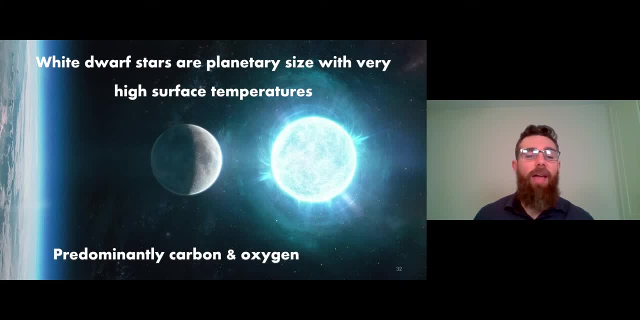 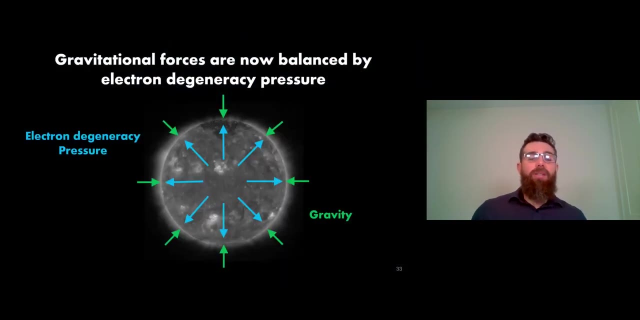 so terrestrial planet size As a general rule, and they're mostly made of carbon and oxygen, because that's what's left behind from a solar-like star once it's finished the end of its fusion, part of its life. Now here, what's holding them together? because they've actually collapsed, and 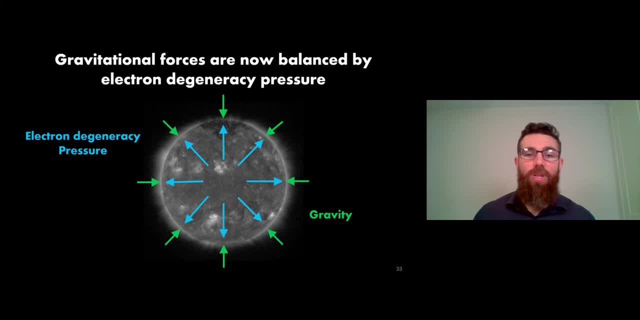 you've now got this degenerate star from a solar system. You've got the much bigger star because star, which means that there was then nothing, There's no outward pressure holding the star together. You've got that gravitational force which is still there. So that gravitational 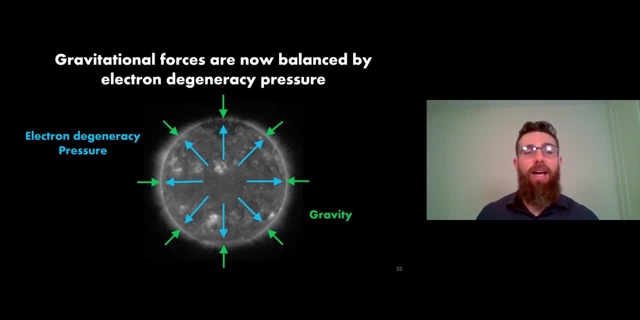 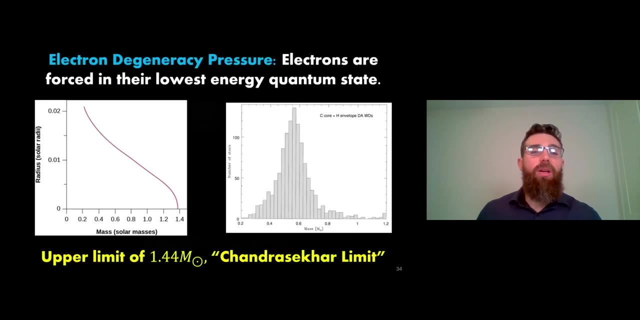 force collapses the star, And the only thing supporting it now is this electron degeneracy pressure. So this is where the electrons are forced into their ground state. This then causes a pressure that can support itself against the gravitational forces. So here you've actually got the distributions of known white dwarfs. So on the right-hand side, 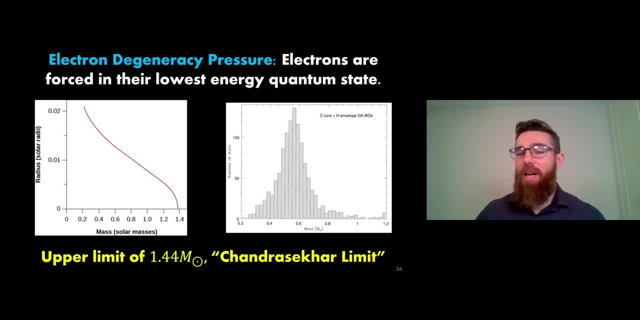 you can see that actually, if you look at white dwarfs, they have a typical peak around 0.6 solar masses. Now it's worth noting that because it's the central core of the star that's left behind, it doesn't mean that the star originally was 0.6 solar masses. It would have been a bit bigger. 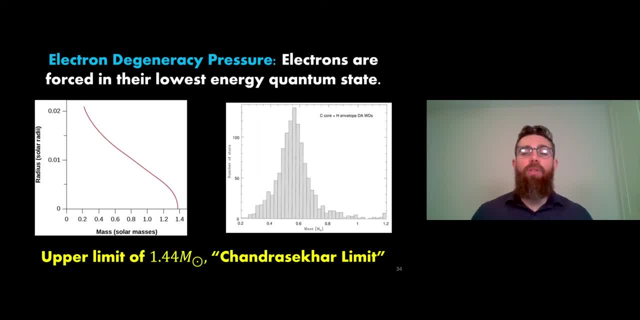 So it would have been probably bigger than the Sun. But this distribution is most likely down to the fact that it's not the center of the star, It's the center of the star itself. So you can see the effect of the stars that were, you know, populating the universe at the time. 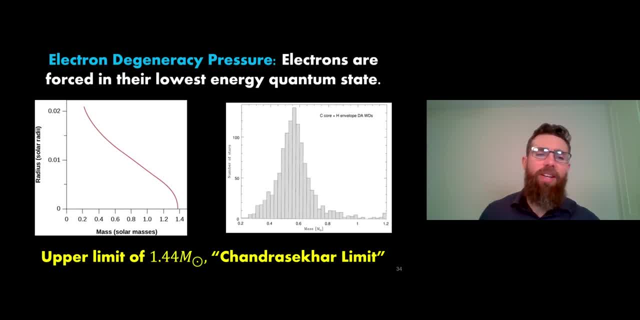 as opposed to the white dwarfs themselves. And then on the left-hand side you can see how the radius of the white dwarf changes as the mass increases, to the point when you get to about 1.4 solar masses, and then you get a sudden shrinking again or collapse. 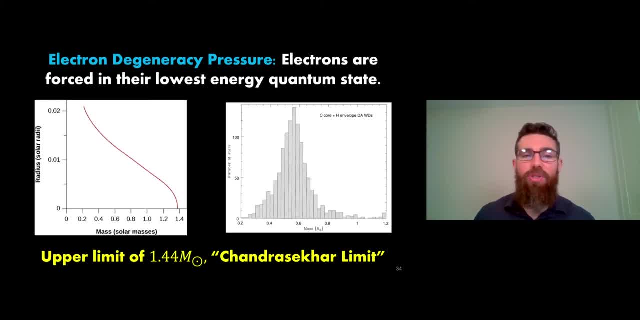 And there's an upper limit which is about 1.44 solar masses, And at that point there the electron degeneracy pressure is not able to support against the gravitational forces and you get a further collapse. So you have this limit again: 1.44 solar masses. That's the upper limit for the mass of a. 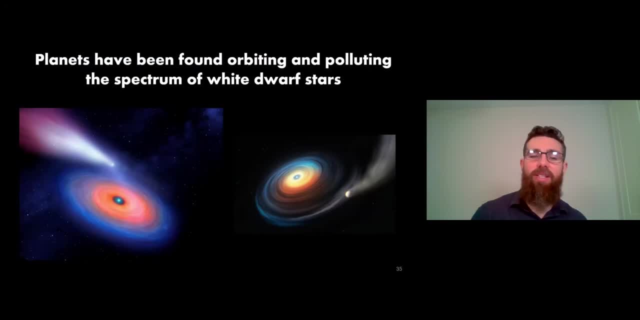 white dwarf. Now, the interesting thing actually is that planets have been found orbiting and also polluting the spectrum of white dwarf stars. So if we've got planets orbiting them, even if they're being destroyed, it means they have survived the planetary nebula phase, the red giant phase. 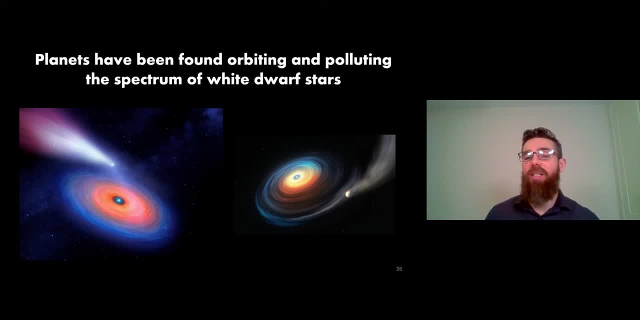 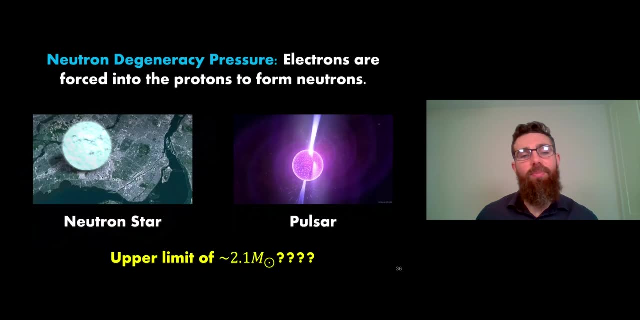 To then be still orbiting the white dwarf, which is quite interesting and exciting, really, because it has implications for our own solar system. going forward Now, if your star is larger than you know the Sun, or a bit larger than that, 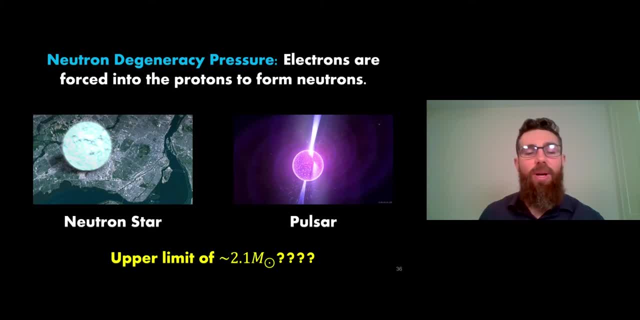 more so, or larger than that- 1.4 solar masses, when it's actually ended its life, then you're going to end up with a neutron star or pulsar. Now, they're kind of one and the same thing. so all pulsars are neutron stars, but not all neutron stars are pulsars, and it could be down. 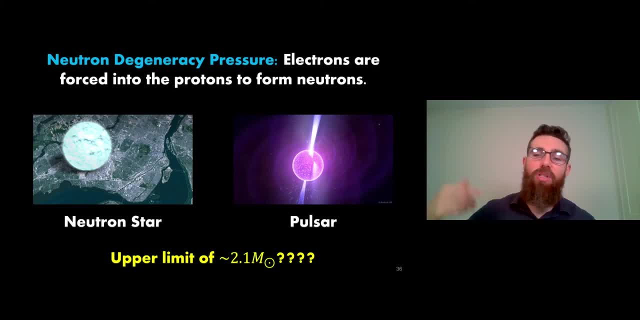 to the way that we observe them. So these pulsars have a beam of light, not light. they have a beam that we can pick up and we get a pulse every rotation, or we get two every rotation, depending on how it's actually orientated. But at this point here these are held up against. 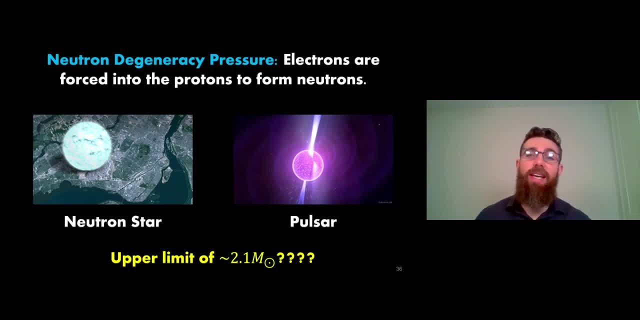 the gravitational force by neutron degeneracy pressure instead, and this is where your electrons are then forced into the protons to form neutrons, And it's thought that there's an upper limit of about 2.1 solar masses. Again, there's a bit of uncertainty there and we don't have a lot of observations at that. 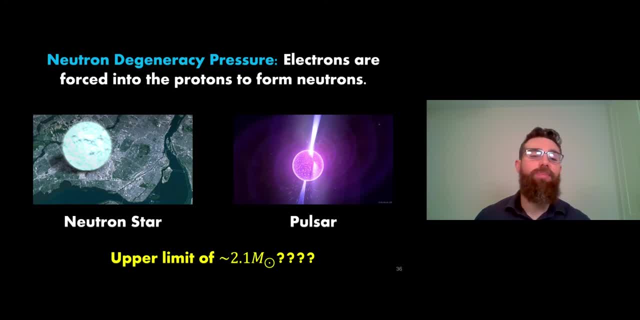 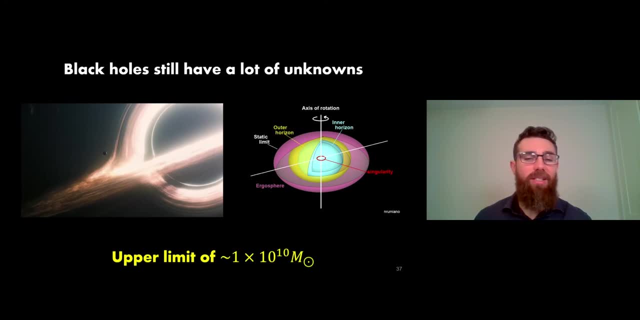 upper limit as well. so it's mostly theoretical. And then if you have larger stellar remnants than that, then you're likely going to get a black hole. Now there's a lot of unknowns about black holes because you can't just directly observe them. 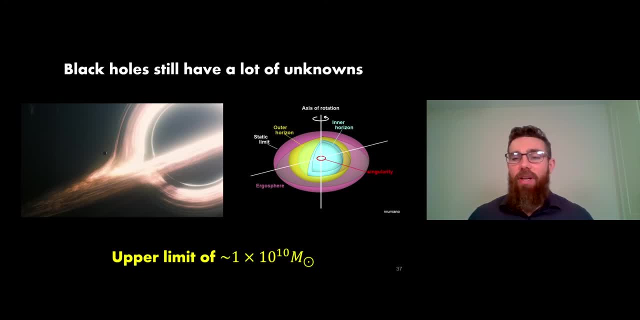 but they do have this event horizon. and if you have a rotating black hole On the right hand side, I've got a bit of a diagram there. so you end up with multiple horizons. you have an outer horizon, inner horizon. 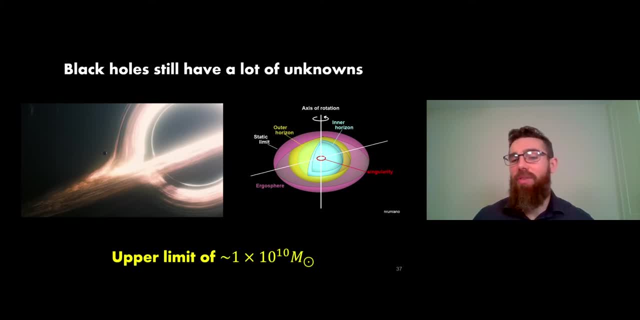 you then also have this ergosphere, which is where you're able to take rotational energy out of the black hole as well, But I'll not mention much about them. The only thing worth noting is that there is an upper limit on black holes, or thought to be, and it's about 10 to the 10th solar mass. 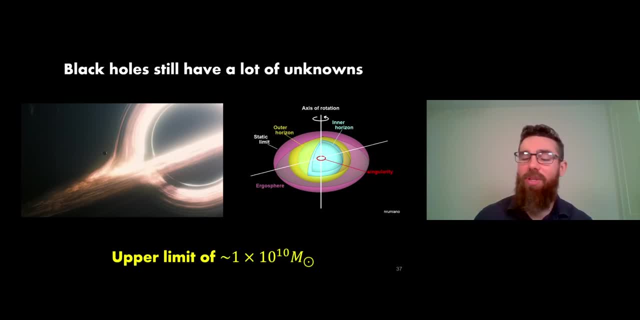 solar masses. These are not stellar black holes, which is probably worth noting, And you can have black holes in a whole range of masses. Stellar black holes have to be formed from the depth of a star, so they can have a very particular range, But these supermassive black holes are in the 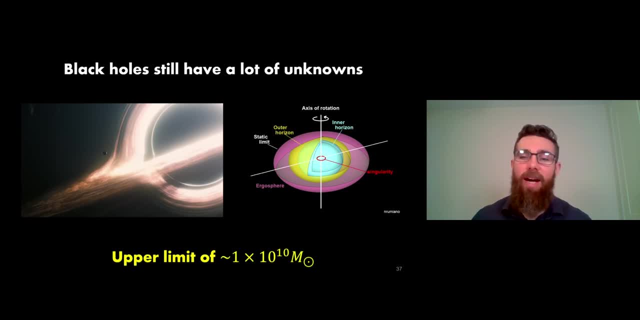 centre of galaxies and they almost self-limit their mass because when they get so large they're drawing in gas from all over the galaxy. It's funnelled in, and when they take so much gas you get star formation occurring in that gas. That then causes a bit of a feedback. 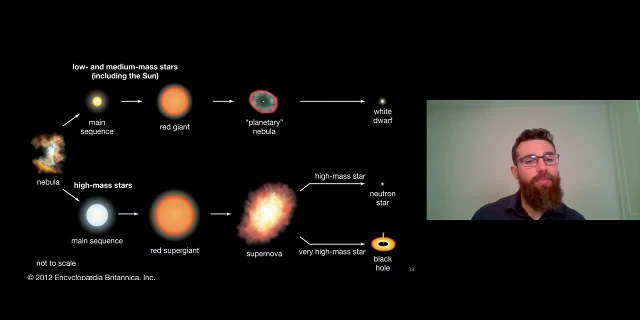 and it limits the amount that they can actually grow by. So if you want to have a look at the general overview of stellar evolution, it's purely down to mass really. They're starting mass. So low-mass stars they go. nebula, main sequence. 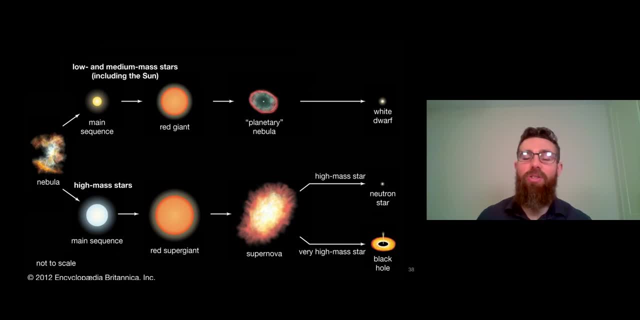 red giant, planetary nebula, white dwarf- That's kind of what our Sun will do, And then the larger ones will do a similar sort of thing, but they will have a supernova and they'll end up with a neutron star. 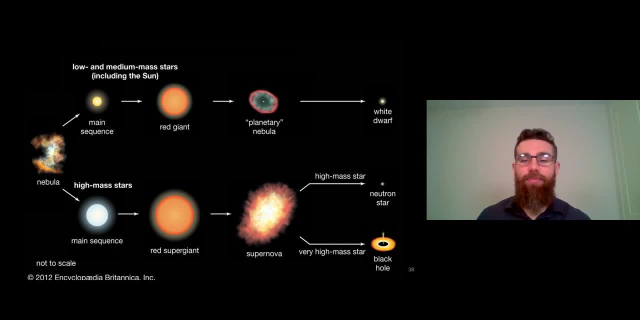 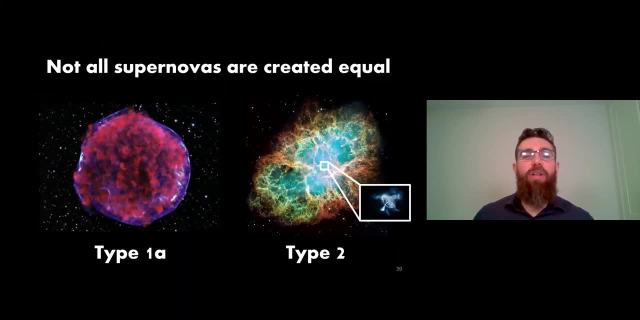 or a black hole, depending on their mass, And it's just purely down to how large or massive the star is. Now, it's worth noting that not all supernovas are created equal, So you have type 1 and type 2.. There's a lot of subcategories in there, and the two I've picked out here to show. 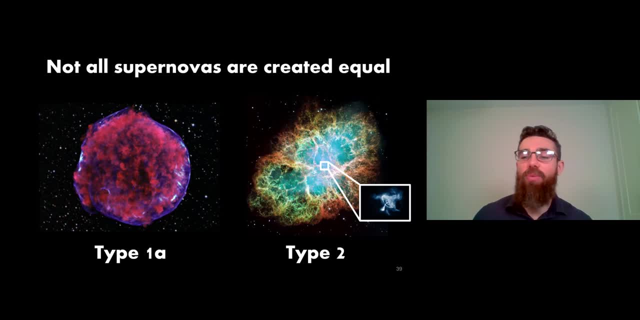 you is the type 1a and the type 2.. So the type 2 is from the depth of a large star and the type 2 is a singular event with a single star, And then a type 1a is actually from a binary system of a white. 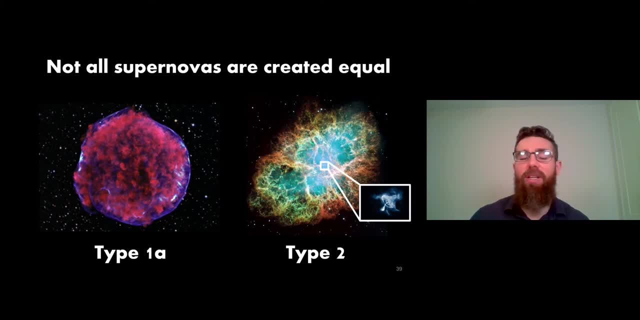 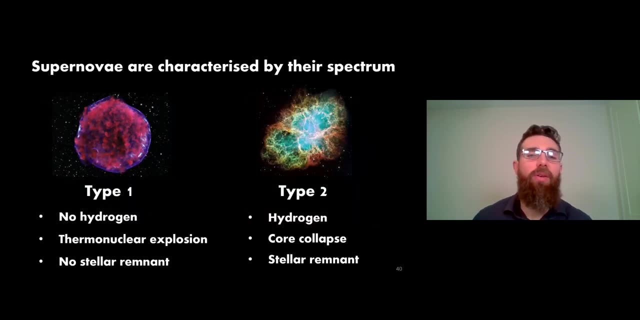 dwarf and a red giant star And it's a very specific supernova And they're quite different. So they're mostly characterized by their spectrum. So type 1, you don't get any hydrogen, It's a thermonuclear explosion and you don't get a stellar remnant at the end, So the whole star. 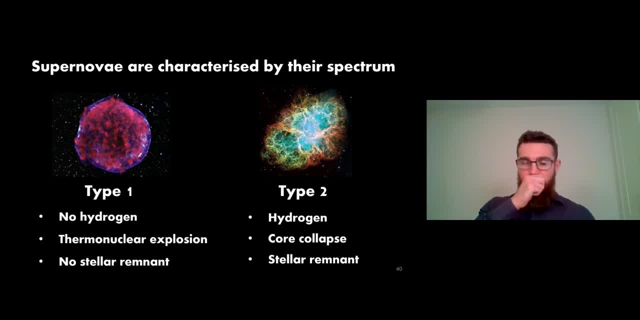 environment is destroyed- Type 2,. you do see hydrogen in the spectrum. It's from the core collapse of a large star at the end of its life, And you do end up with a stellar remnant, most likely a neutron star or a black. 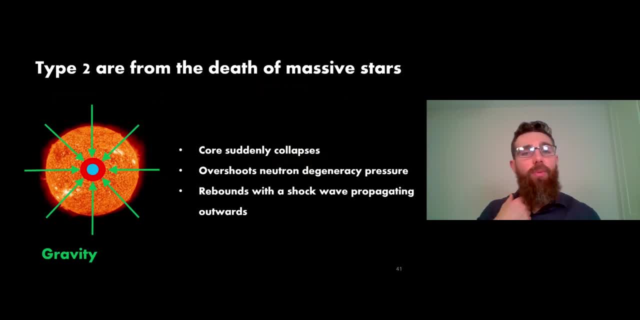 hole, Now the type 2, this is from your depth of the massive star. Your core suddenly collapses when your fusion ceases at the center, So there's no longer that outward pressure supporting the gravitational force. So what happens is you get a sudden collapse. 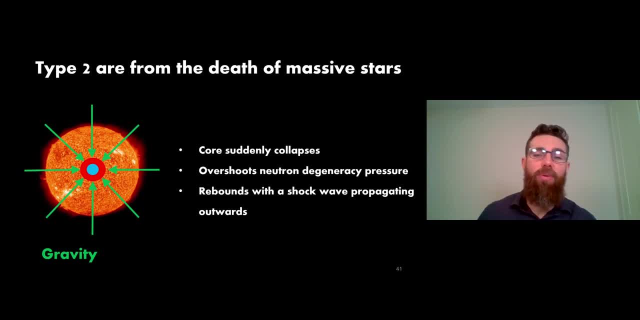 It overshoots this neutron degeneracy pressure and you get a rebound with a shock wave that then propagates outwards through all the outer layers And that then is the basis for a supernova or type 2 supernova. They're not all the same, because it depends on their mass and their composition. 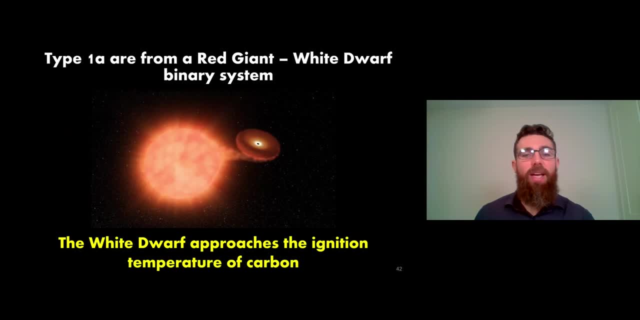 and things like that, Type 1a. so here you've actually got a red giant- white dwarf binary system And what happens is the white dwarf is drawing material off the red giant And that white dwarf then approaches the ignition And it's a supernova. And it's a supernova, And it's a. 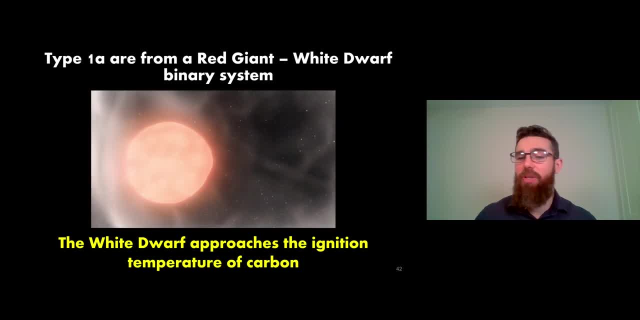 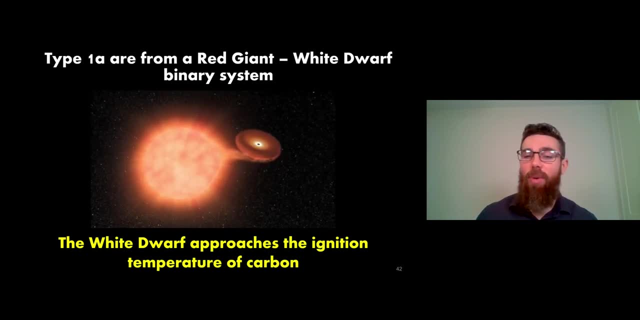 station temperature of carbon And then it just detonates And you get a type 1a supernova. And it always happens at around about 1.4 solar masses, that upper limit for a white dwarf. So once you hit that mass limit you get a runaway detonation of the carbon that it's made of. 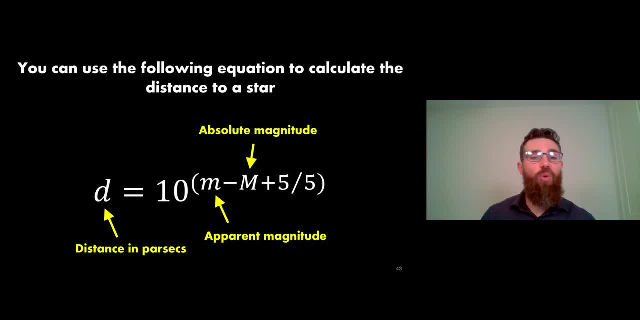 Now the good thing about the type 1a is they supposedly all happen at the same mass, so the same energy, Therefore the same energy. So you get a runaway detonation of the same luminosity, same magnitude, And you can then use them to work a distance to the star. So we 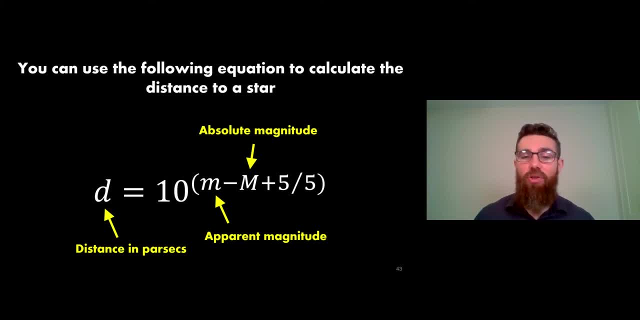 can use this equation here. So you have the apparent magnitude, which is what we would measure. That's what we would observe. The absolute magnitude is what it would be from some set distance. So the absolute magnitude would always be the same. The apparent magnitude would change. 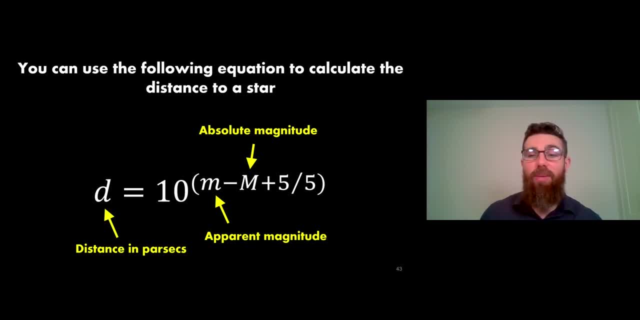 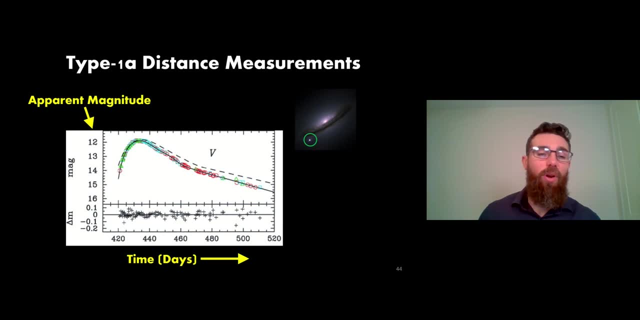 depending on how far away it would be, And then we can work a distance to it in parsecs. So here you've actually got the light curve of a type 1a supernova And you can see that the supernova. so that plot there just shows you how bright it gets from when it first occurs. 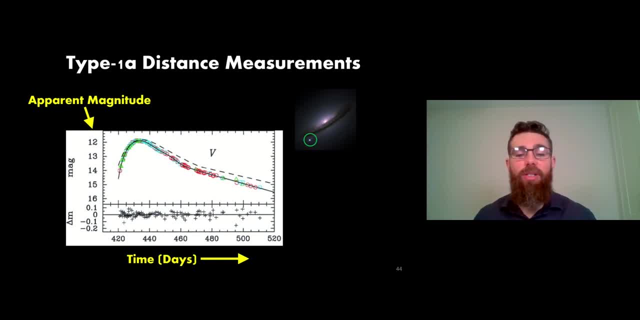 And you've got one occurring in the galaxy on the right there, And they can be quite bright And then over time it will peak in a few days and then it will slowly dim down And the apparent magnitude is on your y-axis And obviously your time is on your x. 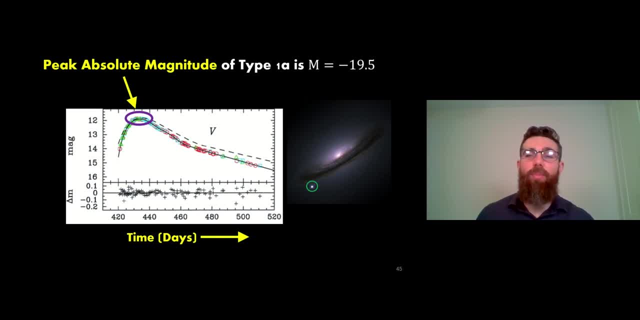 Now the peak absolute magnitude of type 1a is about minus 19.5.. And we can see from the light curve: if we take the peak there, it's around about 12, which would be our apparent magnitude, And if you put that into your equation you can work out a distance to it. 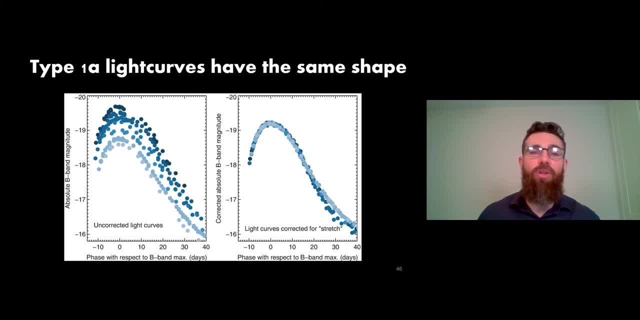 Now the type 1a- light curves pretty much all have the same shape. You might have to do some kind of correction for it, so some stretch, But basically they all have the same shape. Now the type 2s wouldn't necessarily have the same shape because they're not all the same. 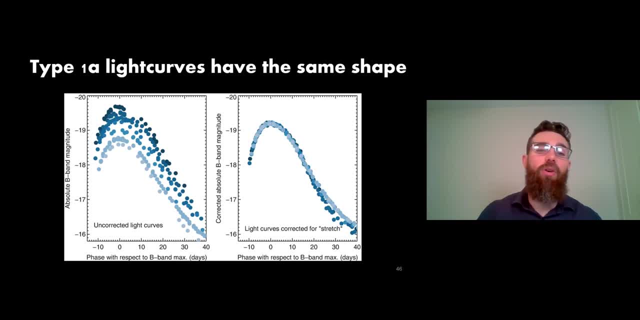 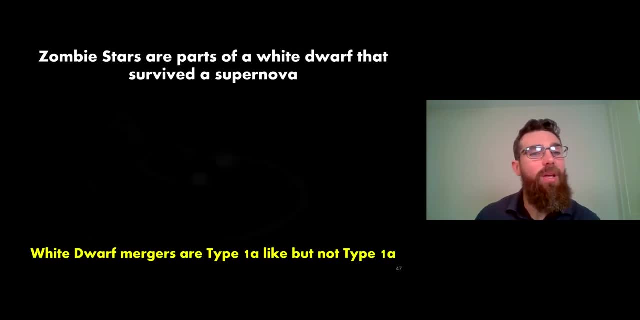 mass. They're not always the same competition Composition, So there are variations there, whereas type 1a should all have this similar shape to the light curve. Now, finally, we just have an example of a type 1a that's not a type 1a. 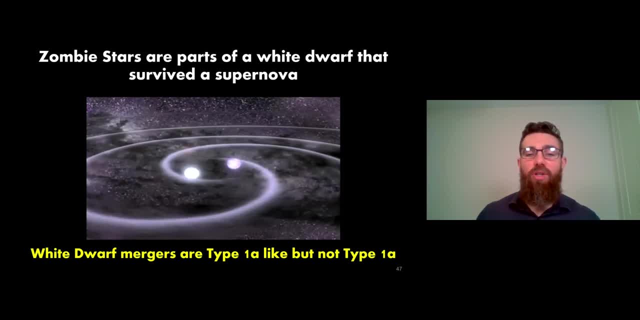 So here you've actually got the merger of two white dwarfs. Now they could have a combined mass that is greater than 1.4 solar masses. So therefore it could appear to be type 1a, but you've actually exceeded.